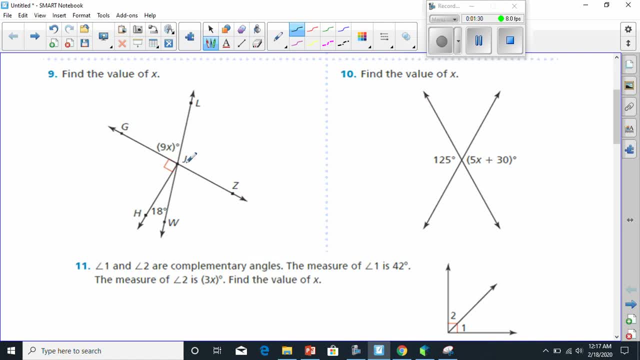 This is nine X, And that's the only X listed here, And so we've got to go ahead and figure out what nine X is. We're going to use all of our property skills to go ahead and figure this one out. First of all, we see that this is a 90 degree angle, So we already know this is 90.. 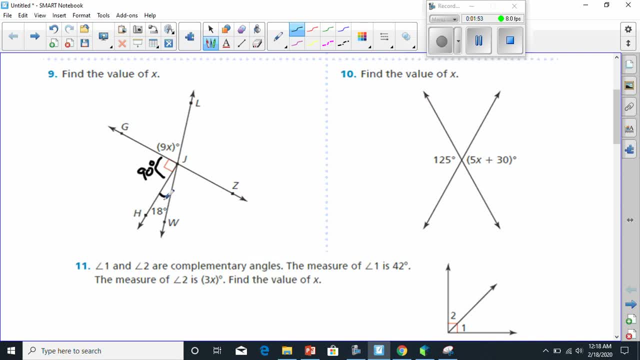 We also know that this angle here is 18 degrees, So we can say this entire piece here: angle G, J, W is going to be 90 plus 18.. And of course that's going to give us 108.. That's very significant because now that we know this is 108 and we know every straight line is 180 degrees. 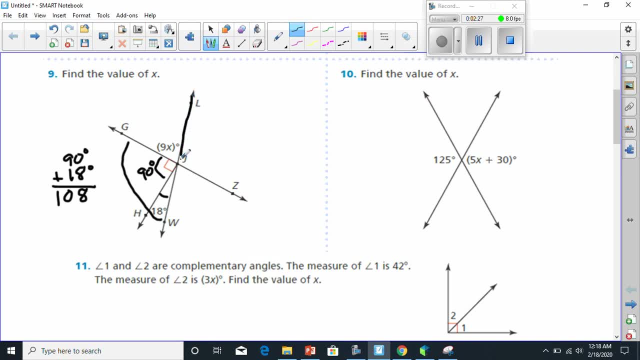 We can look at the line that goes from L to W here, And if that's 180 degrees, well then this 90 plus 18, we should be able to subtract it from 180 to find out what this angle is. So now we've got 180 minus 108. 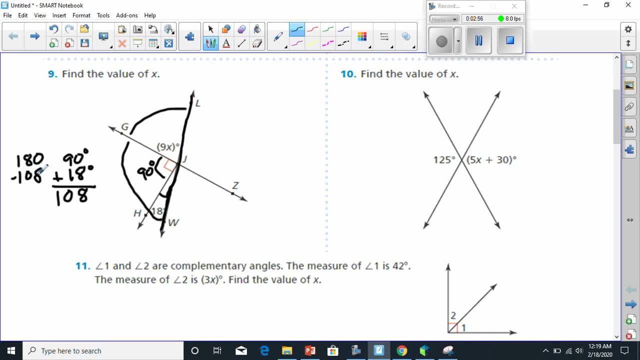 Okay, And that's going to give us two. We borrowed one from here, So I'll leave a seven. So that means this angle is 72 degrees. Now we also know this angle is nine times X. So we can say that nine times X is going to be equal to 72 degrees. 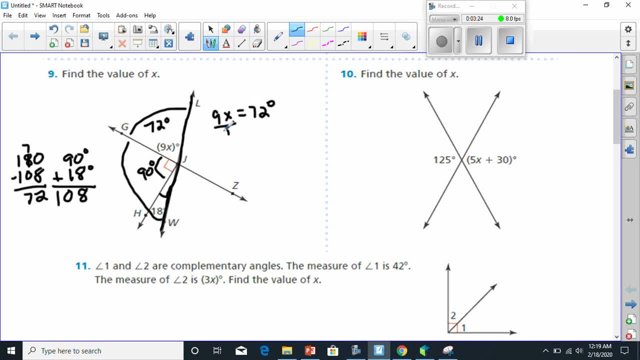 And if that's true, we can use the properties of that, Use the properties of division here, Isolate X by itself. Whatever, I divide from one side, I divide from the other, And now X is going to leave us with. well, nine times eight is 72.. 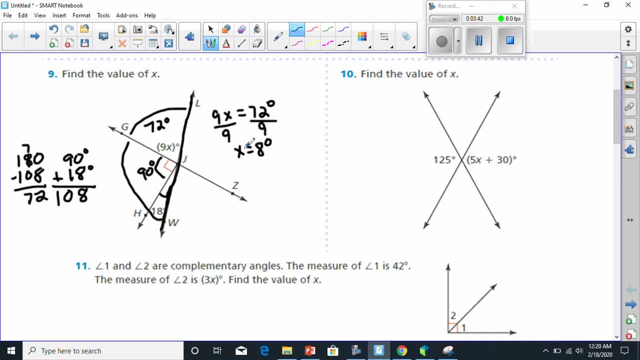 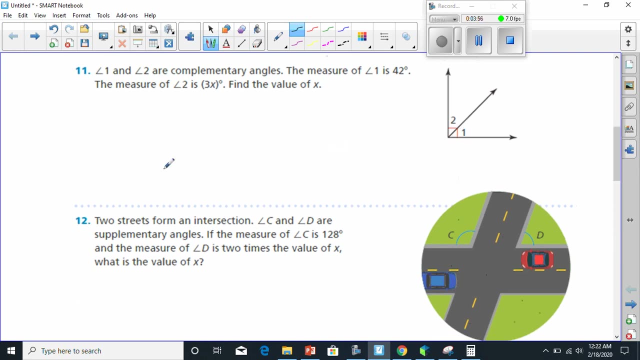 So this must be eight degrees, or X is eight degrees, And that solves number nine. Let's go ahead and move down now to number 11.. 11 says the angle one and angle two are complementary angles, which means these angles will equal 90 degrees. 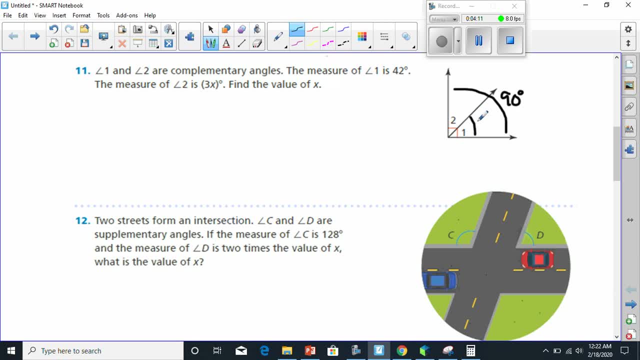 The measure of one is 42. So this is 42.. Number two is 3X. Well, that means this is 3X. Find the value of X. Well, we know that 90 degrees is going to be equal to 42 degrees plus 3X. 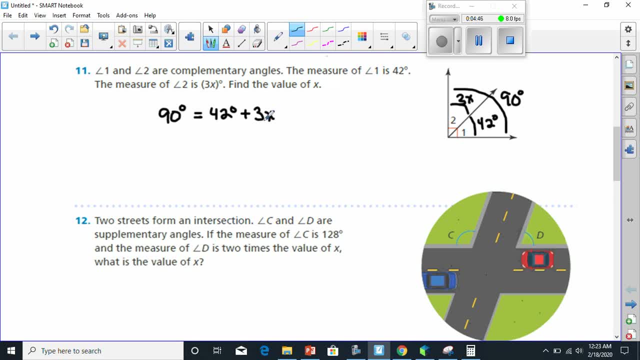 And we solve this by using the same properties, Properties we use for two-step equations. First, we're going to isolate the variable by getting rid of the numbers using our properties of subtraction. When we do that, we see we have 3X left over. 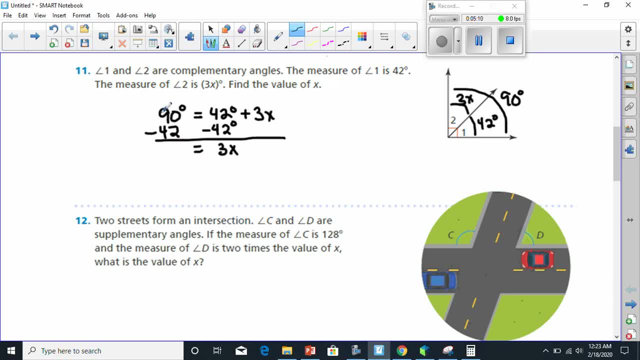 All right, And then, well, we're going to have to borrow one from here, which is going to leave us 48. And now that I know that I can- I can, I'm sorry- 48. I can use my properties of division to isolate X by itself by dividing three away from it. 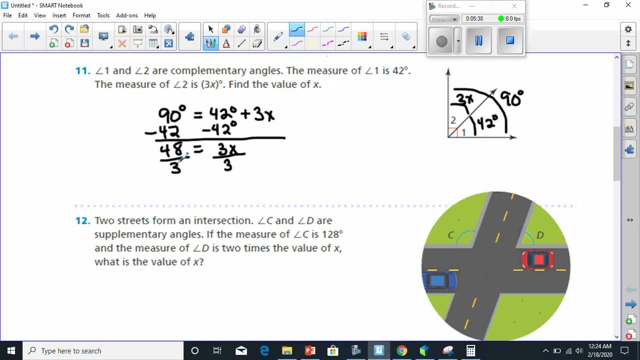 And whatever I divide from one, I divide from the other. And now I have to say: what is 48 divided by three? Well, 48 divided by three will give us 16.. So 16 is X. Okay, Let's see. 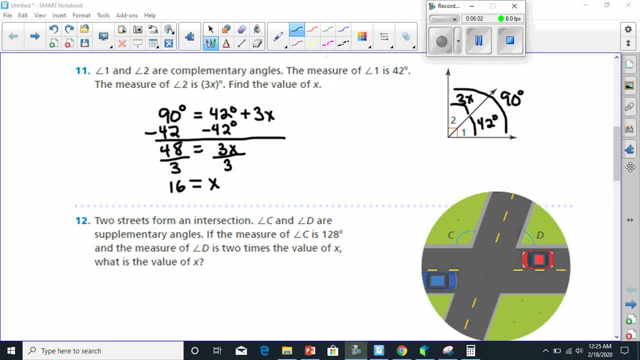 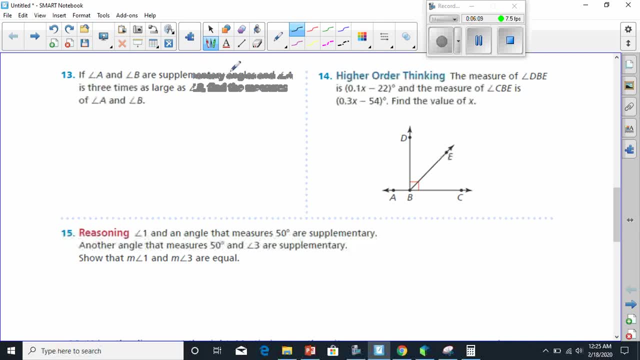 I think I've got number 13. now I'm going to scroll down here to number 13.. It says that angle A and angle B are supplementary angles. Well, that means that angle A And angle B Have to equal 180 degrees. 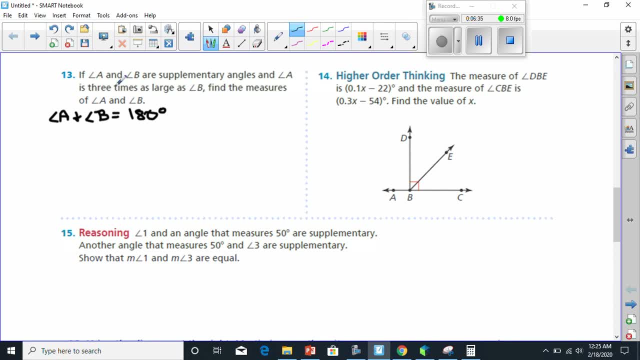 Next, we can see this as an angle A is three times as large as angle B. Well, that means angle A. Well, if it's three times As large as angle B. Well, hold on. We could simply write this to say: we can use substitution here. 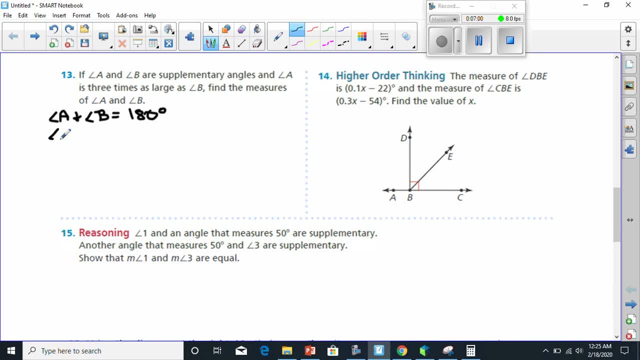 Let's see If angle A Equals Three. I said three times Angle B Up here We can Use substitution And we can put that three Angle B's. I'm going to rewrite this: Three Angle B's. 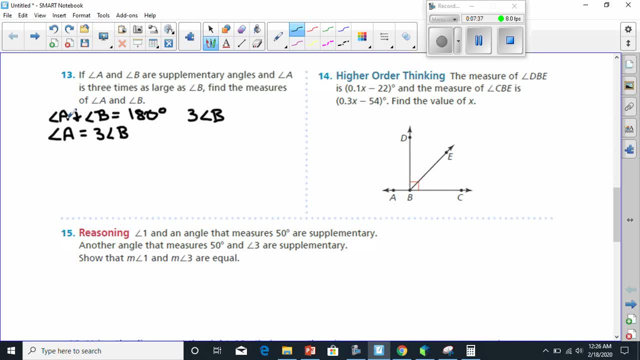 All right. It says angle A is equal to three angle B's. So we're going to replace angle here, A in this equation with three angle B's, Plus Angle B Has got to be equal to 180.. This should help us because that means that four angle B's right. 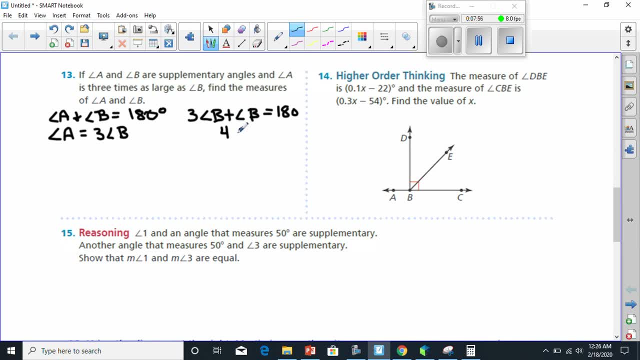 Three plus one equals four. angle B's Equal 180.. Let's see how this can help us in the future. So find the measure of angle A and B. Well, this isn't that hard, Um. Find the measure of B. 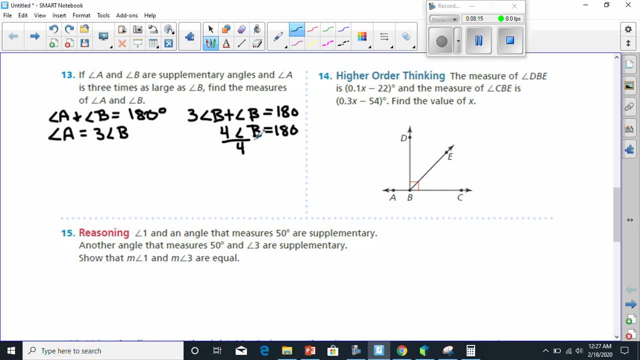 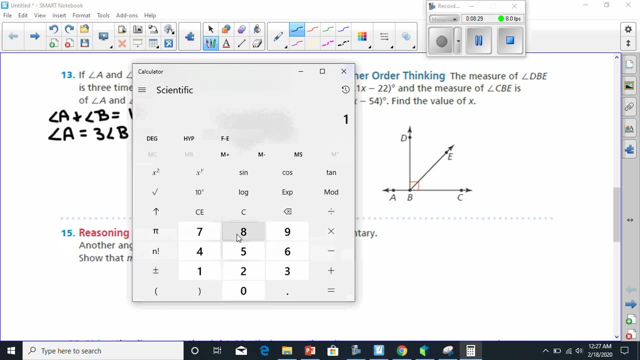 If four angles B equal 180.. I can divide four away, Leaving angle B by itself. Whatever I divide from one side, I have to divide from the other side. I have 180 divided by four, And If I take 180.. 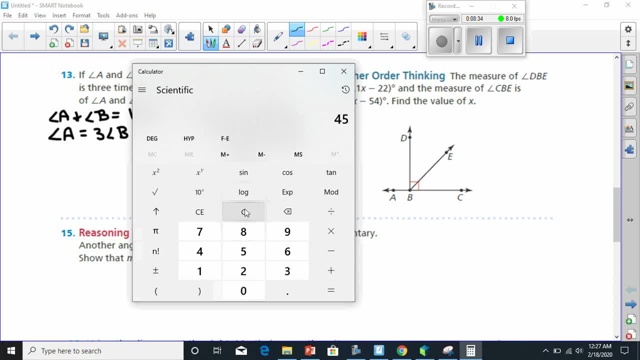 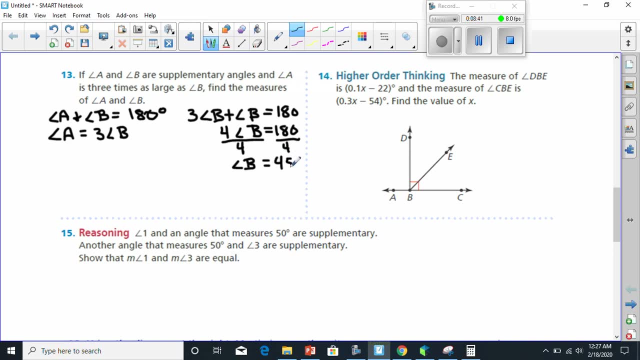 And divide it by four, That gives me 45. So that means angle B is 45 degrees. Now they're saying: Find angle A as well. Well, let's go back over here. If angle A equals three angle B's. 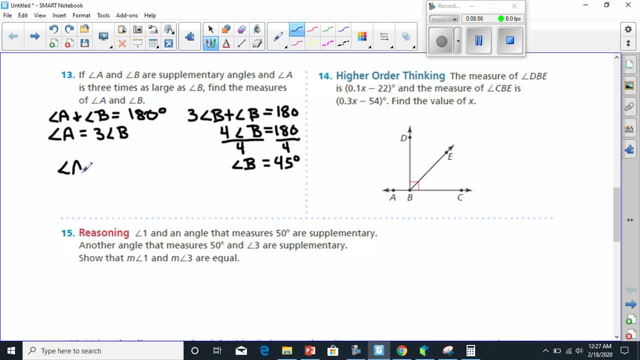 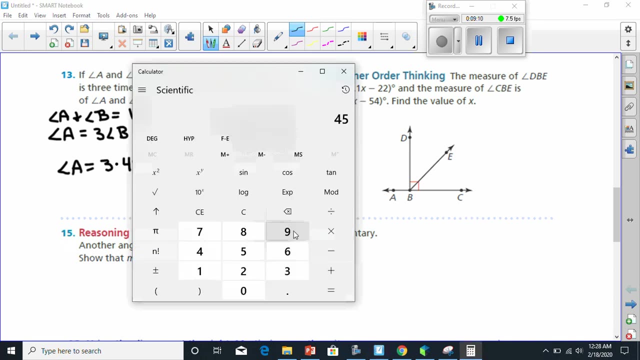 Then that would mean that angle A- We can rewrite this again- Well, angle B is 45 degrees, So that would be three Times 45 degrees, And now we can simply say: What is 45 times three, That's going to give us 135.. 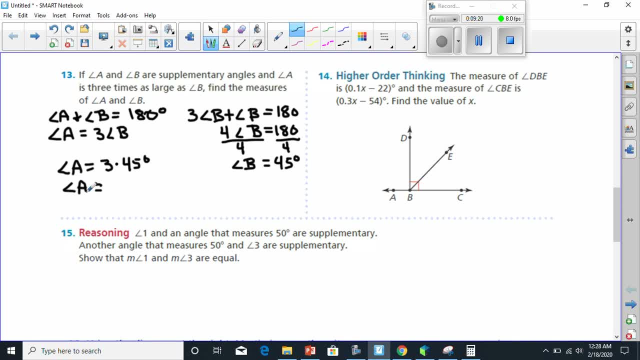 So angle A must be 135.. All right, Now that makes sense, Because 135 plus 45. Remember we said that angle A and B has to equal 180.. So 135.. Plus one or plus 45.. Do this a little simpler. 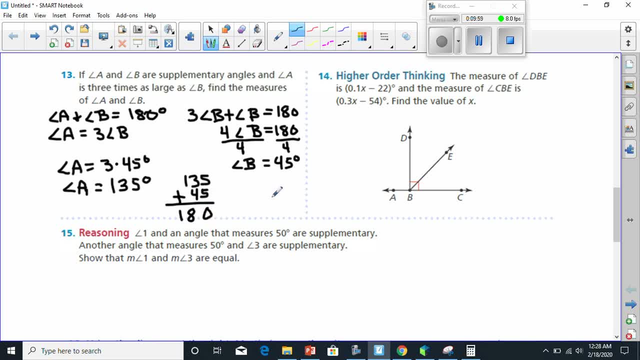 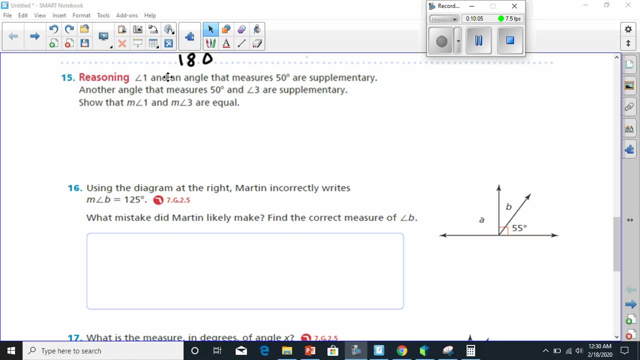 Equals 180.. All right, We're off to number 15 now. Okay, Number 15 says Angle one and angle And an angle. Excuse me, Number one and an angle That measure 50 degrees are supplementary, So we know the angle one. 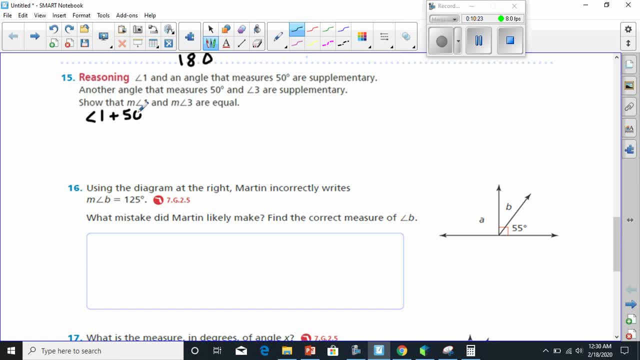 Plus 50 degrees. We don't know what angle it is, But we do know it's 50 degrees Is going to be equal to 180.. And another angle That measures 50 degrees: Okay, And angle three: Okay. 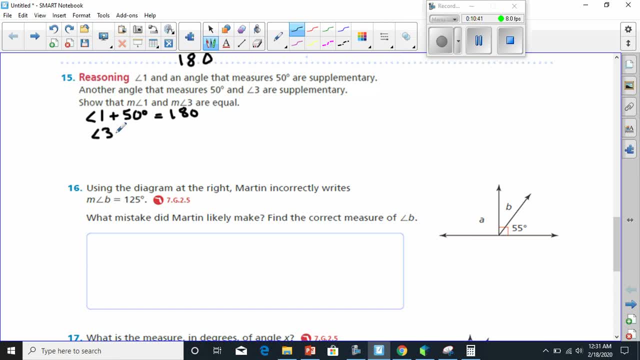 So this would be angle three And another angle Equals 50 degrees, Also supplementary, So they're also equal in 180.. Show that number one and three are equal. This is pretty easy. If I solve this problem here, It's going to go ahead and give me. 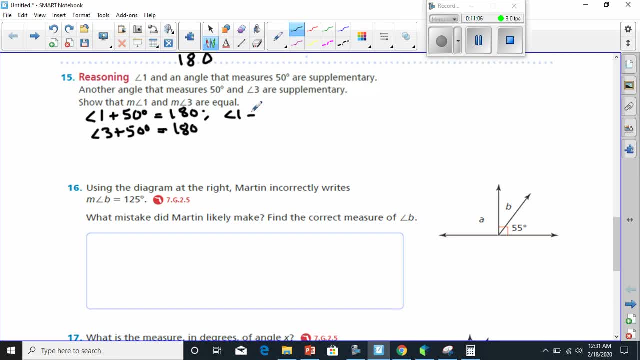 Angle one Is equal To 180.. Minus 50. And I really should say degrees, I guess. So let's see, That means That angle C, Or angle one, Must equal 180 minus 50.. That's 130.. 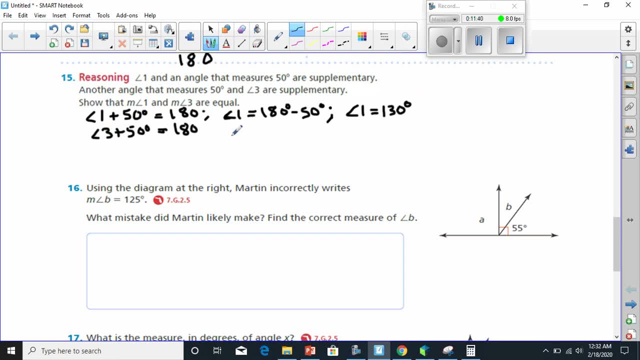 If we solve for Three, It should be no different, because If angle three Is also equal to 180.. Minus 50.. We're using the Properties of subtraction. Remember, I need to get One by itself, So I'll subtract 50 here. 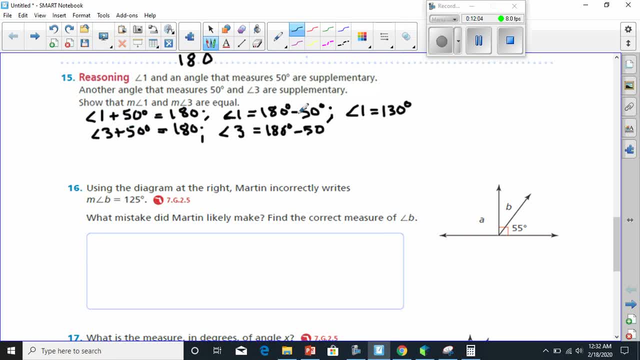 And I'll also subtract 50 here. Whatever I subtract from one side, I'm subtracting from the other side, And that means that Angle three Also has to equal 180. Because 180 minus 50.. I'm sorry, 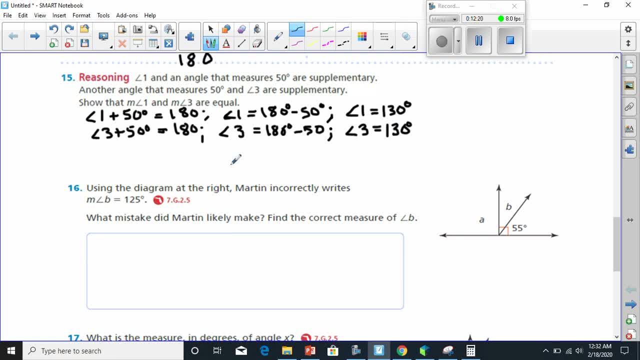 It has to equal 130.. Not 180.. There we go: Angles one And angles three Equal 100.. I'm writing through. I don't want them to say Like you have to add them together, So I got to. 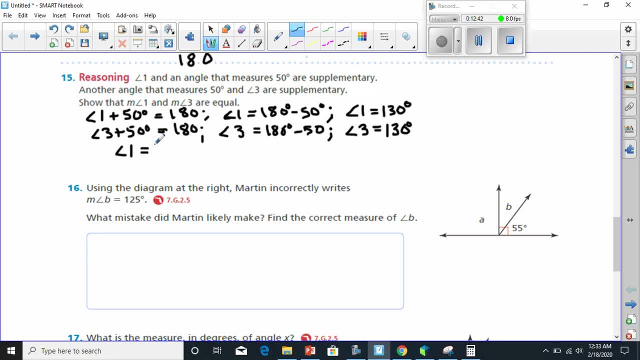 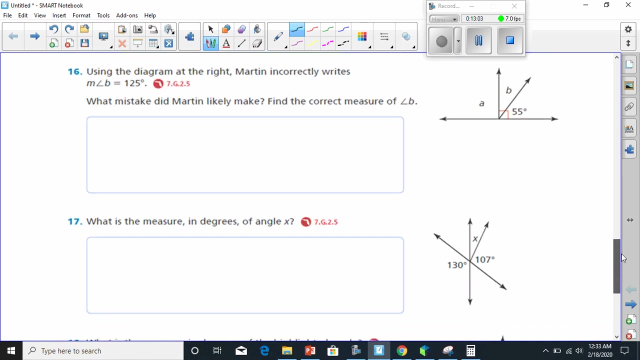 Correctly put this in: Angle one Equals 130.. And Angle three Equals 130 degrees. All right, Moving down to That is how we Show that they're equal. We're moving down to number 17 now. 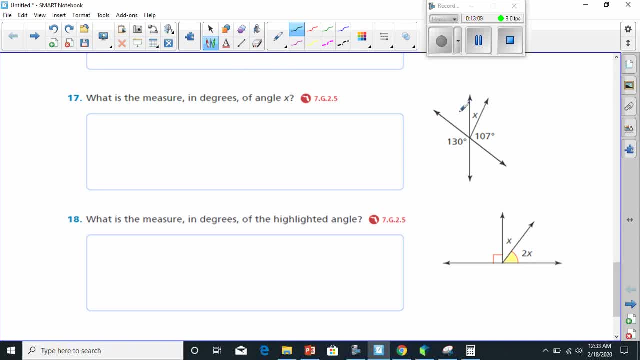 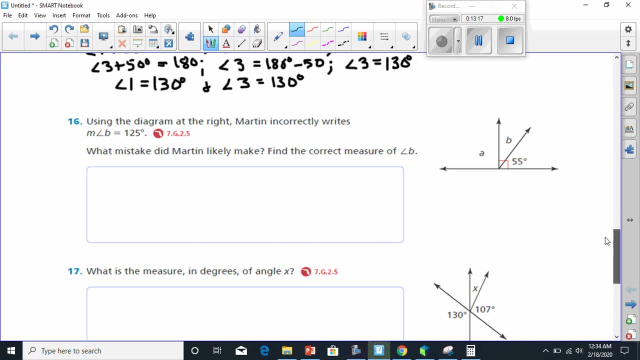 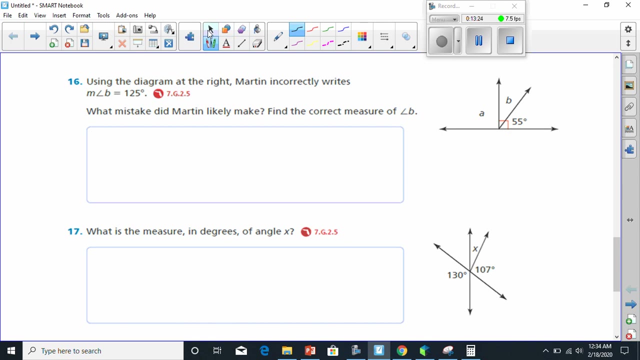 Says: what is the measure in degrees of angle X? Or if I solve for X here And I double checked and realized that Number 15 was the last one We were going to be doing. 1617 and 18 were not a part of the homework. 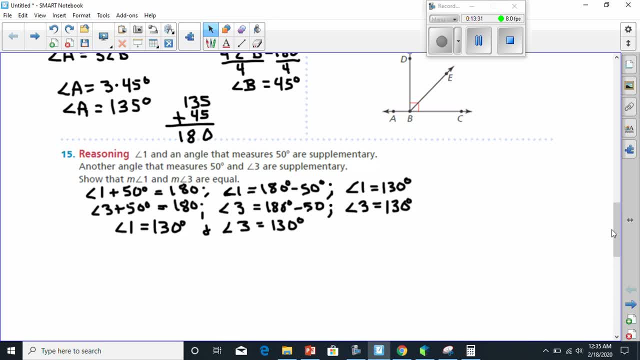 So I'm taking them off there. 15 was your last one, So I guess I'm done And good luck with the ones that you had. I'll see you in class.